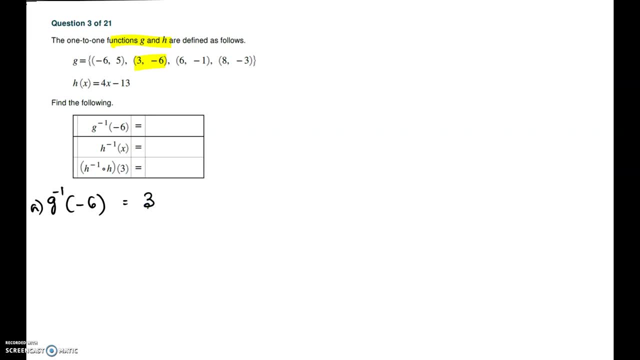 So it is g. So this is g inverse of negative. 6 is 3.. The second part we have to find out: h inverse of x. we are given h of x. h of x is given to be 4x minus 13.. 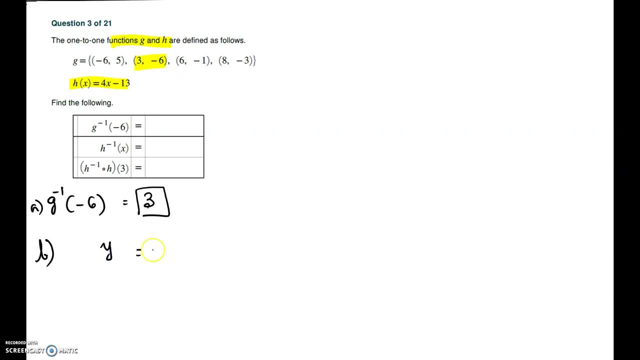 So we have a few steps here. We will first change the h of x to y, y equal to 4x minus 13,. that is step 1.. So we are changing the h of x, We are rewriting h of x as y. 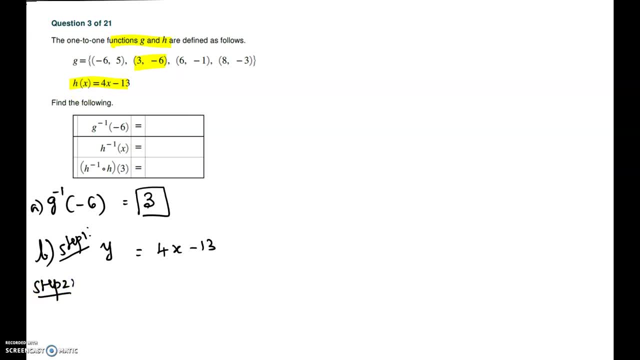 Then in step 2, you will switch x and y, So interchange the roles of x and y, Meaning write y as x and x as y. Next we are going to solve for y. Step 3 is to solve for y, So for y minus 13, equal to x. 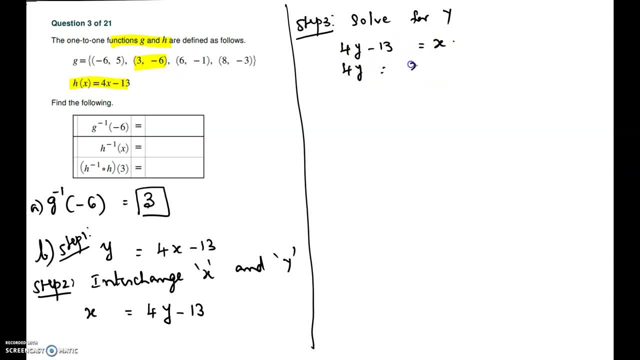 So for y you move the negative 13 to the other side. that will become positive 13. Then you divide by 4 both sides, So you will have now y equal to 1 fourth of x plus 13 over 4.. 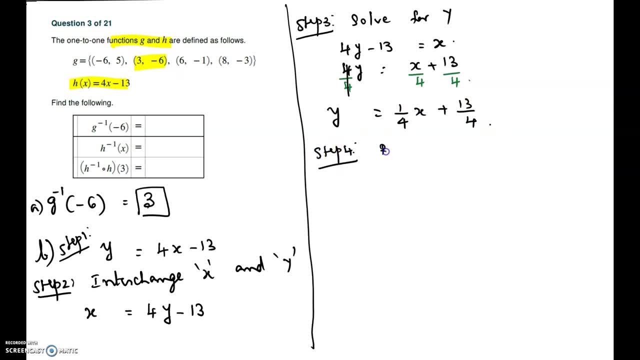 The last step is to change rewrite the y as h inverse of x. So we have to write h inverse of x equal to 1 fourth of x plus 13 over 4.. And the third part is to find h inverse of x equal to 1 fourth of x plus 13 over 4.. 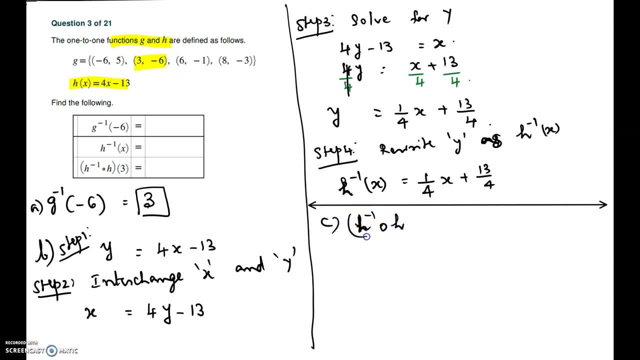 So we have to write h inverse of x equal to 1 fourth of x plus 13 over 4.. So we have to write h inverse of x equal to 1 fourth of x plus 13 over 4.. That is the last part. 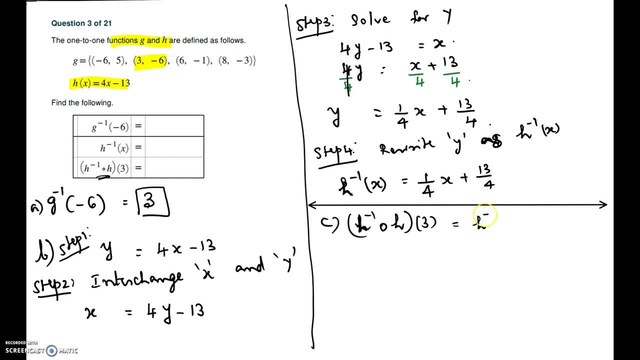 So, using composite functions definition, it is h inverse of h at 3.. So you have to go from inside out. we have to first evaluate h of 3, keeping the outside function as is. So, which is h inverse, we are keeping it as is.